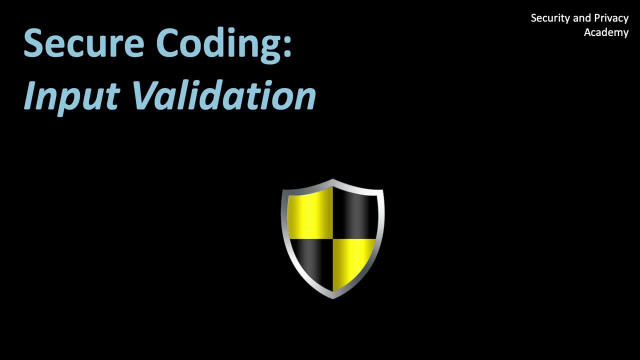 Hello and welcome to my YouTube channel dedicated to security and privacy. In this video, we will explore the critical topic of input validation and why it's essential for writing secure code in programming languages like C and PHP. This video is part of a series on secure coding, and make sure to check out other videos in 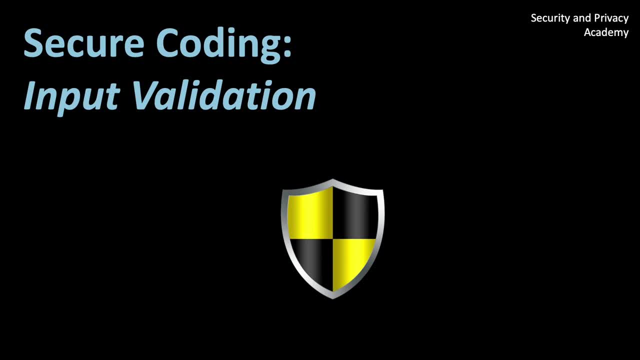 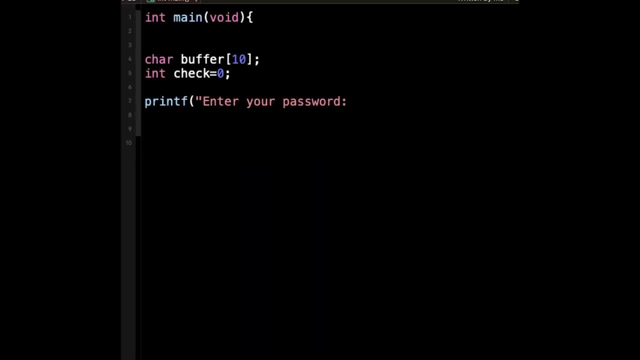 this series. Now let's begin with C programming. One common vulnerability in C is using the gets function to read user input. The gets function reads characters from the standard input until it encounters a newline character, without considering the length of the input or buffer size. 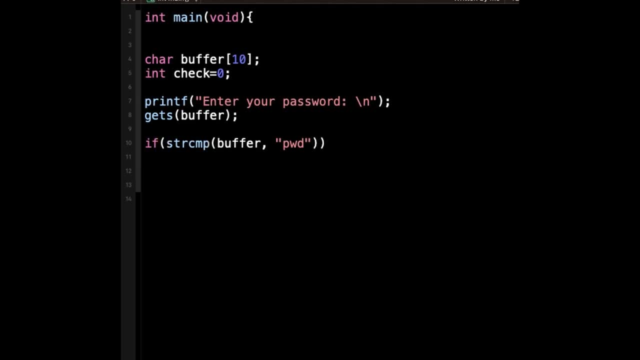 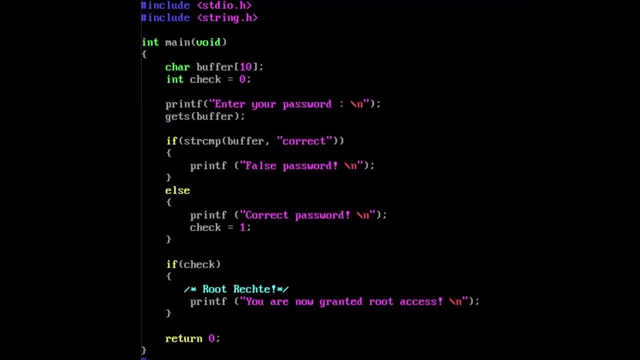 Here's an example that uses gets in order to compare an input string with the actual password. The final program looks like this: You can see that the password is read by the function gets And that if the string comparison yields 0,, which evaluates to false, it shows correct. 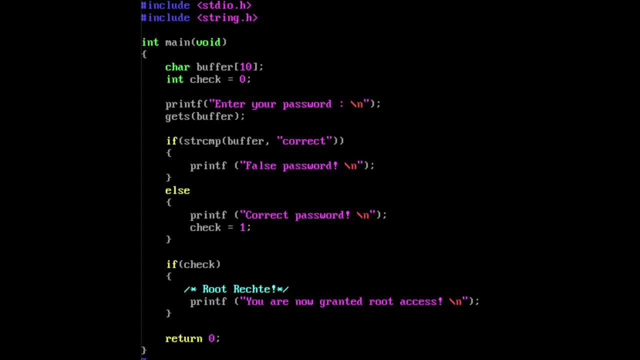 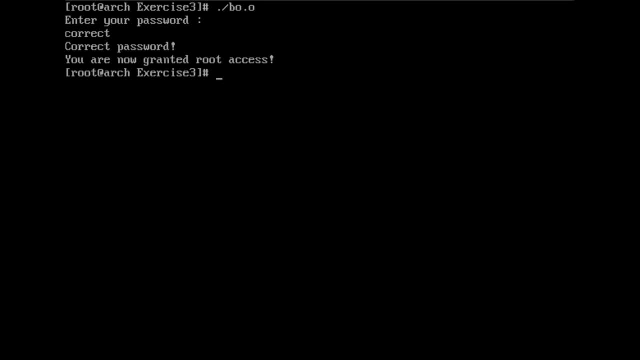 Obviously, using the correct password works, but using a wrong password does not, if it has 10 or less characters. As soon as I enter a password that has more than 10 characters, I overflow the buffer and check is set to any value, but it's not 0, and therefore I'm now root. 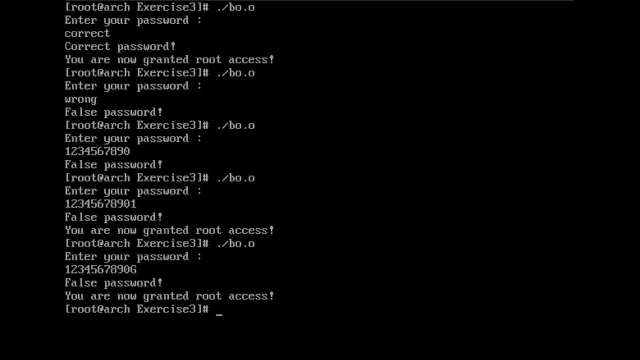 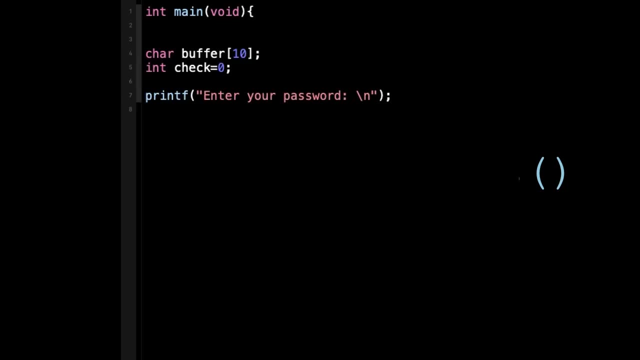 That's real hacking for you Now, obviously it's a very artificial example, but it just serves to illustrate a point. To mitigate this vulnerability, it's crucial to use input validation techniques like fgets. The fgets function reads a specified number of characters from the input stream and stores 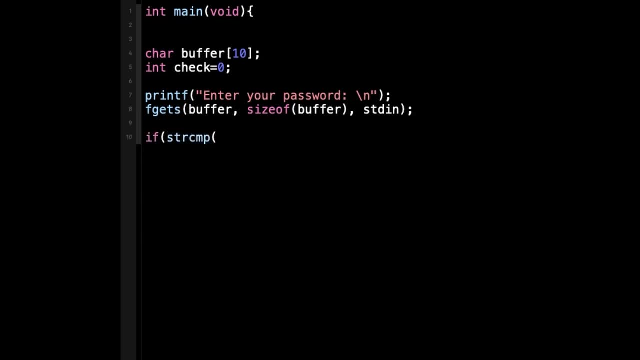 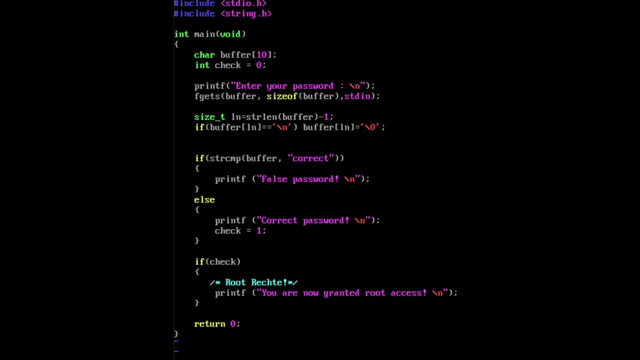 them in a buffer. like gets, However, fgets ensures that the buffer size is not exceeded. By using fgets with the appropriate buffer size, we can prevent buffer overflow vulnerabilities. It ensures that the user input is truncated or rejected If it exceeds a specified number of characters, then the user input is truncated. 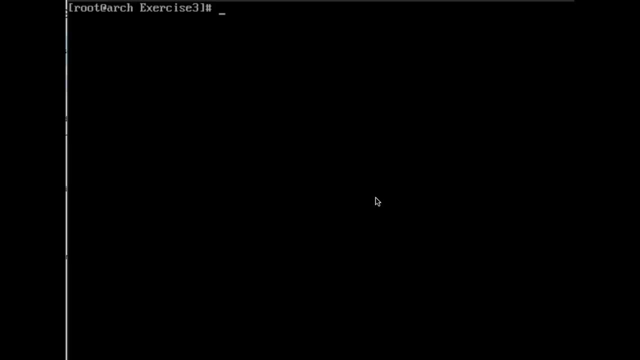 If it exceeds a specified number of characters, then the user input is truncated or rejected. This allows the user to specify the specified length, providing a safer and more secure code implementation. Again, in this case, using the correct password works, A wrong one fails. 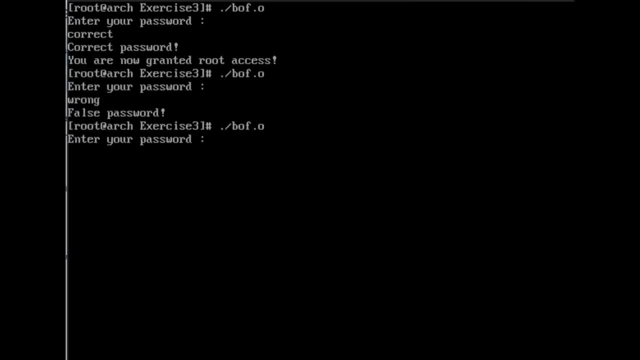 But even using an exceedingly long password, so more than 10 characters, which is still the size of our buffer- it will not overflow the check variable, as fgets checks the bounds of the input and truncates it accordingly. So using fgets is safer than using gets, obviously. 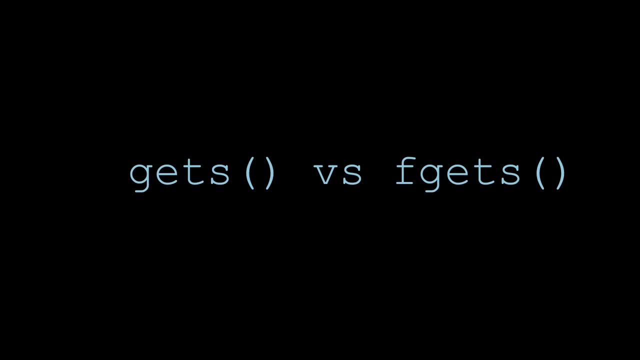 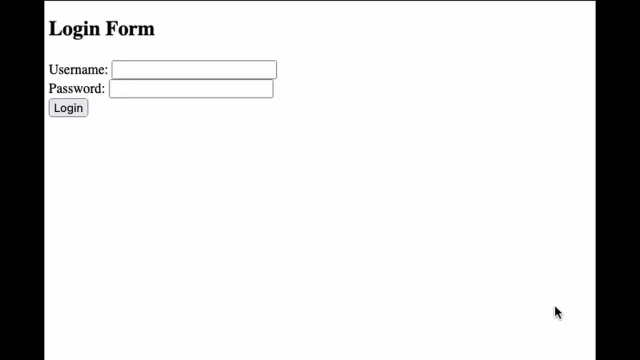 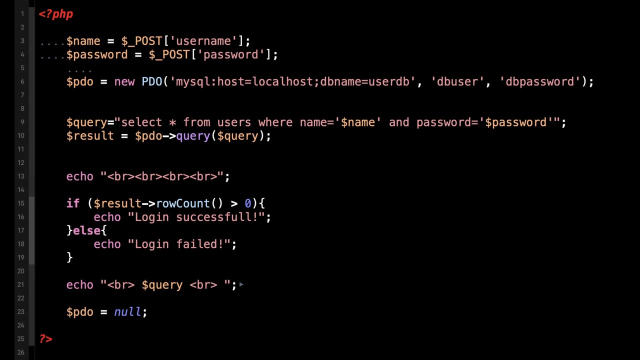 But checking that your input is what you expect it to be is more than just using save function. For the second example, We look at SQL injections. Let's assume we have this username password combo to log into a website. Let's look at the code. This builds the database connection and the query is constructed by the variables handed over by the previous HTML form. 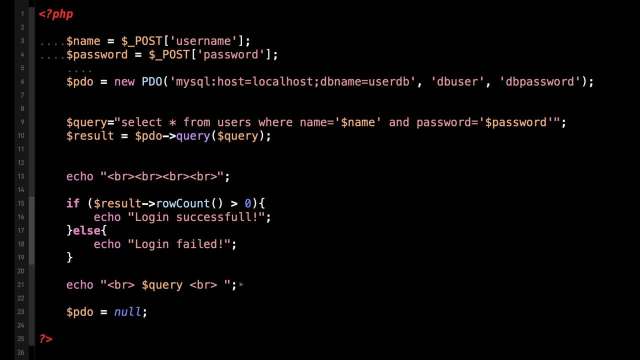 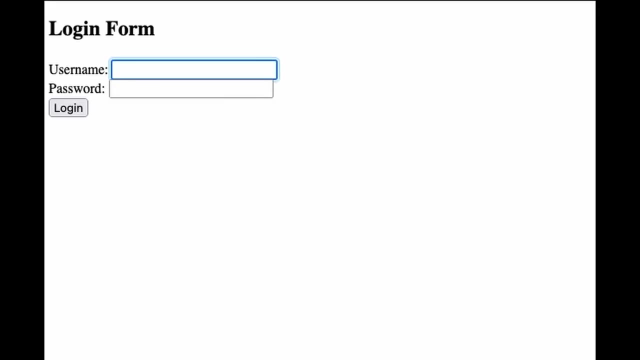 The query is executed and after a couple of breaks- if the result is not zero- we get a successful login. Logically, this approach is sound, since we only get a result if both username and password are correct. Let's see how it works in practice Now. if I enter Alice and her respective password, we get a successful login. 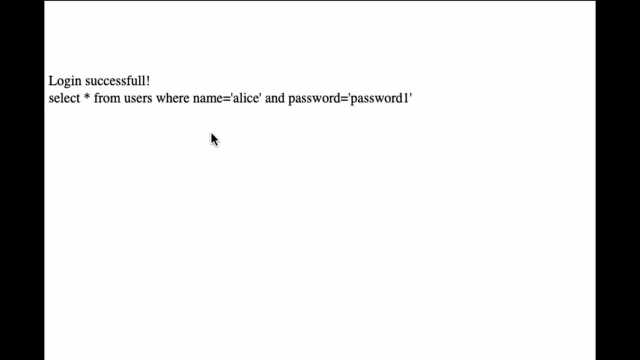 I printed the final query here so we can see what's going on, But obviously don't ever do that in practice. if I enter a wrong password, we see that login fails As expected, since the where statement is no longer true. all fine so far. Now let's look at the SQL injection, which works like this: 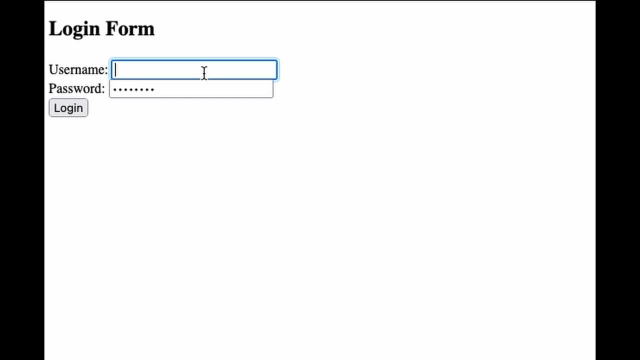 You enter username string and you enter a second operation which is always true, such as 1 equals 1. Finally, the two dashes comment out everything that comes afterwards. We see here the successful login. since the where statement of the SQL query Evaluates to true because 1 equals 1, it doesn't matter what I enter for the username. 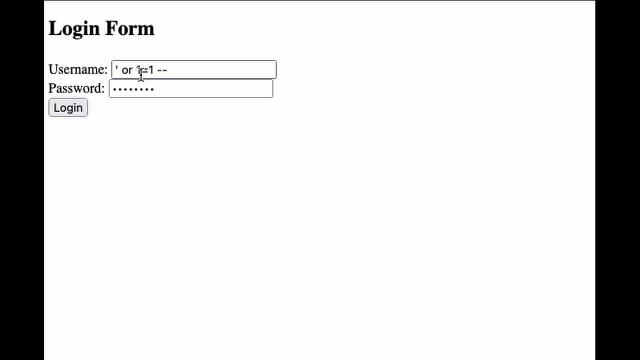 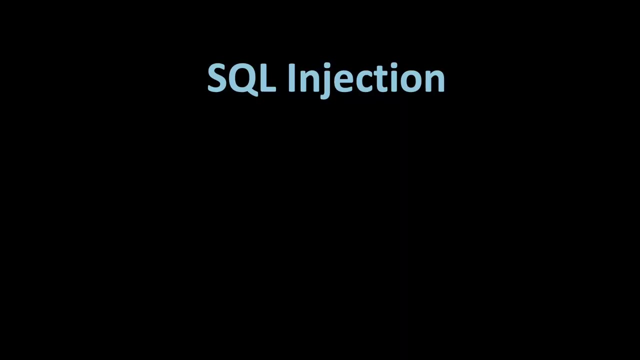 I just need to end the string To inject my 1 equals 1. This is a trivial example again, of course. However, it shows how dangerous it is to not sanitize your inputs. best practice is to use prepared statements, Which means that you don't directly execute SQL queries with provided inputs. but this video is about input validation.